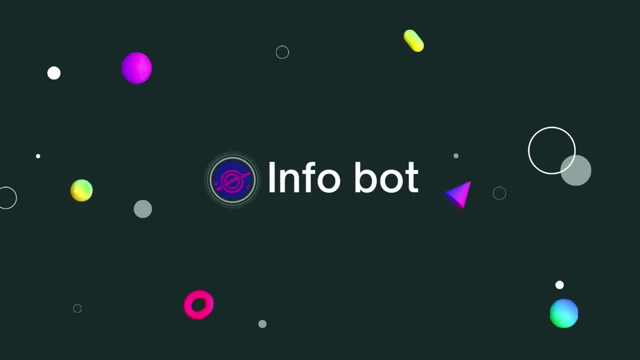 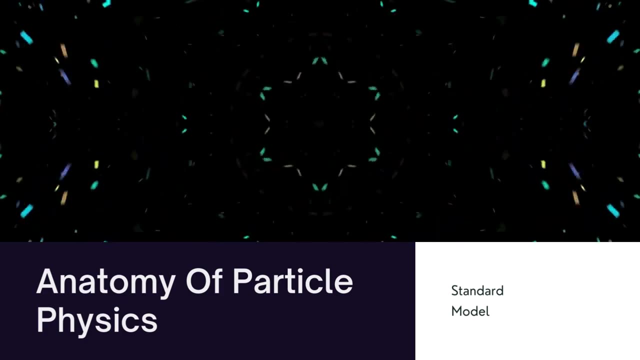 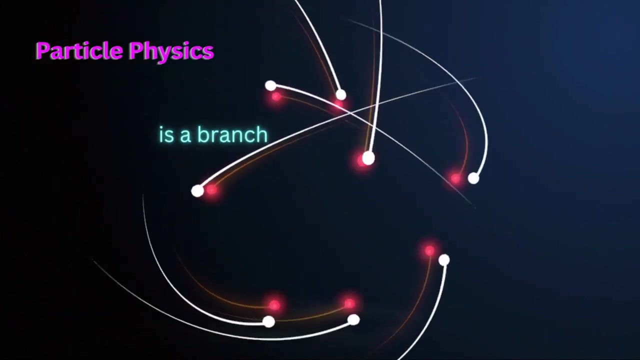 Hello everyone, welcome to my channel, Infobot. Today I'll talk about the anatomy of particle physics. Before start explaining the structure of particle physics, We need to know what particle physics really is. Particle physics, or high energy physics, is a branch of physics that 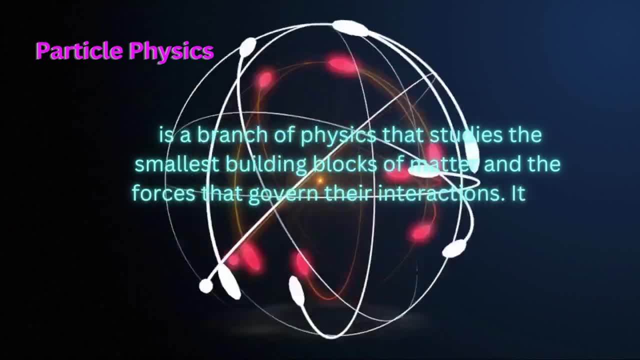 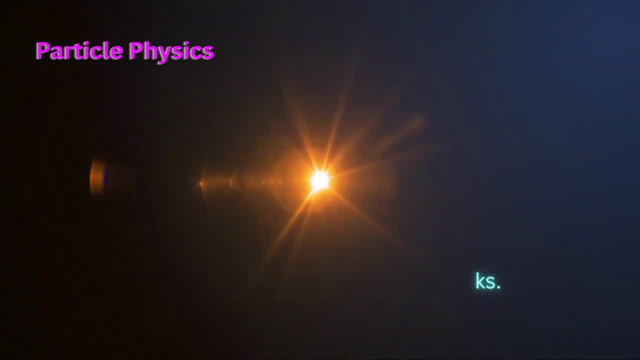 studies the smallest building blocks of matter and the forces that govern their interactions. It is a fundamental field of study that provides us with a deeper understanding of the nature of the universe and how it works. One of the main goals of particle physics is to understand the 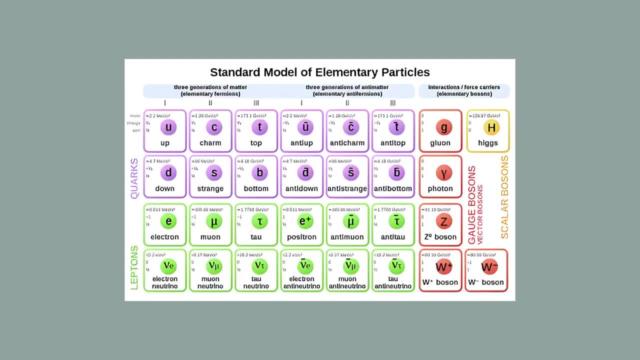 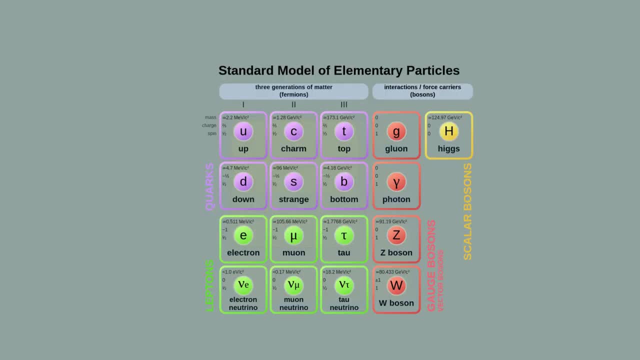 nature of particles and their interactions. I'll only talk about the matter, not their counterparts. antimatter Particles are classified into two categories: bosons and fermions. One of the most significant achievements in particle physics has been the development of the standard model of particle physics, which describes the interactions of all known elementary 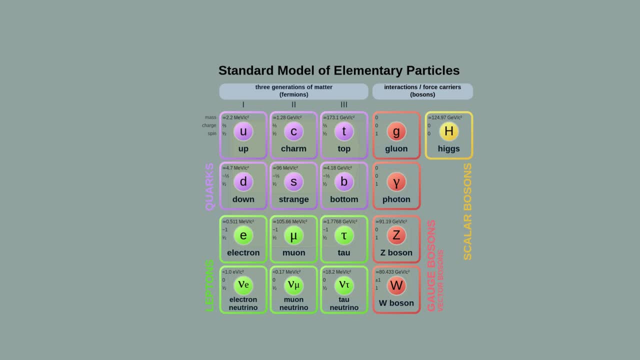 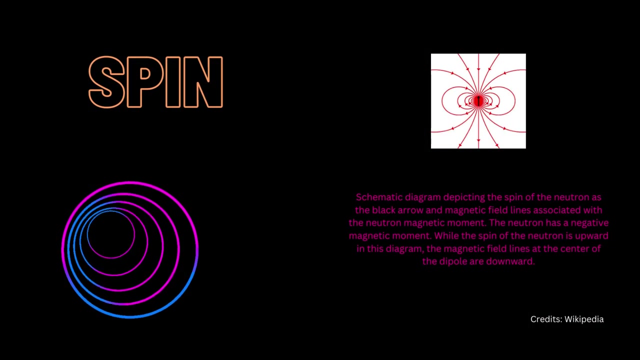 particles and their interactions with the fundamental forces of nature. The standard model consists of three basic building blocks, twelve types of fermions, five types of bosons and the Higgs boson. First, let's start with fermions. Fermions have a property known as spin, which is similar to the intrinsic angular momentum. 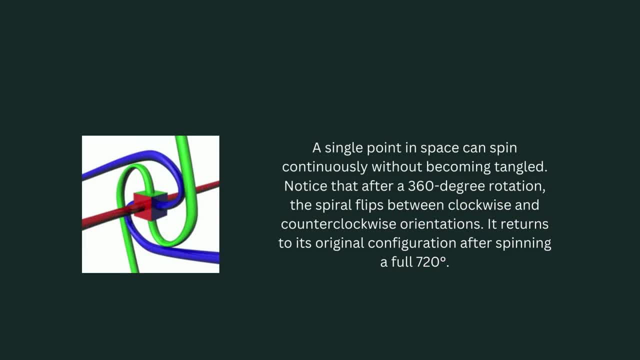 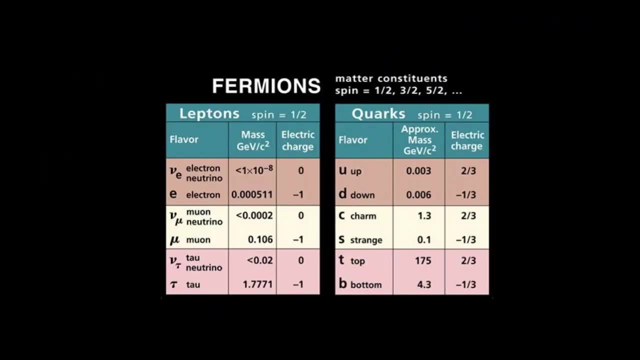 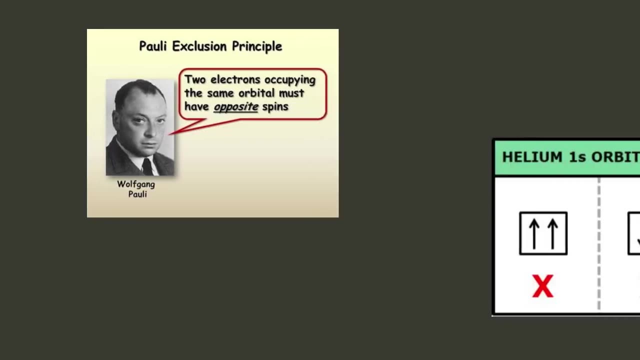 of a particle. Spin is a quantum mechanical property and plays an important role in the behavior of particles. The fermions are divided into two categories: quarks and leptons. They both have a spin of one half, which makes them fermions, and are subject to the Pauli exclusion principle. 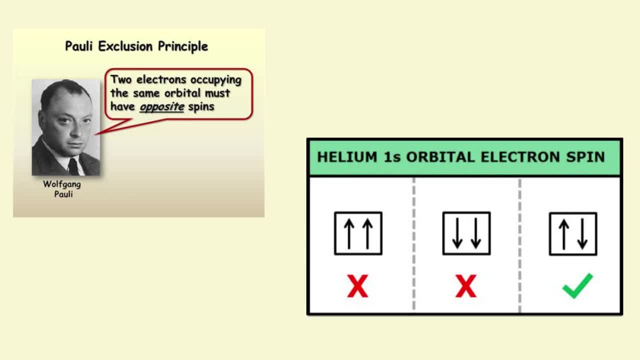 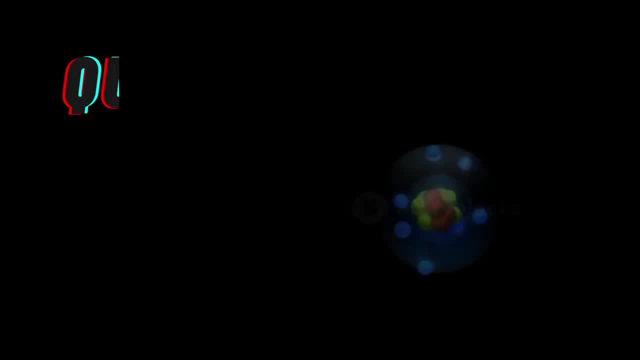 which states that no two fermions can occupy the same quantum state at the same time. The fermions are divided into two categories: quarks and leptons. Quarks: They are the basic components of protons and neutrons, which make up the nucleus of an. 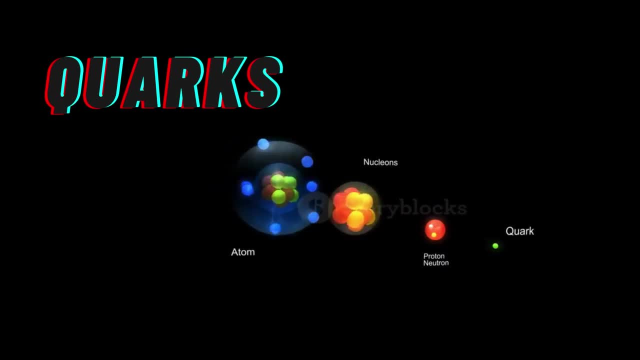 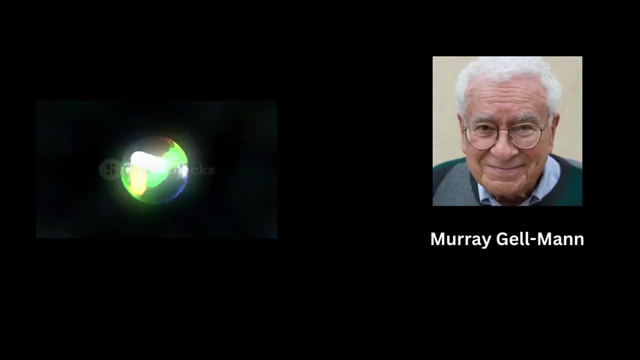 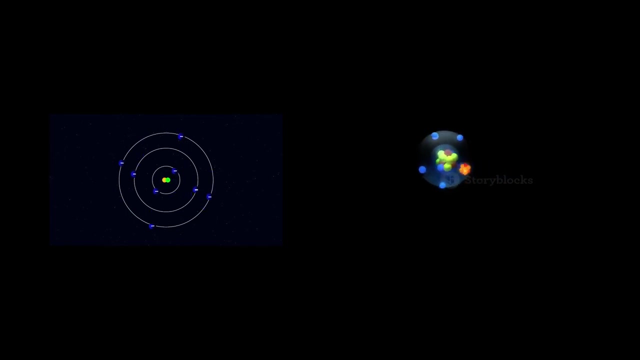 atom Quarks have been the subject of extensive study and have been the key to unlocking many mysteries of particle physics. The theory was proposed by Murray Gelman in 1964, who was awarded the Nobel Prize in Physics in 1969 for his work. Gelman suggested that protons and neutrons were not elementary particles. 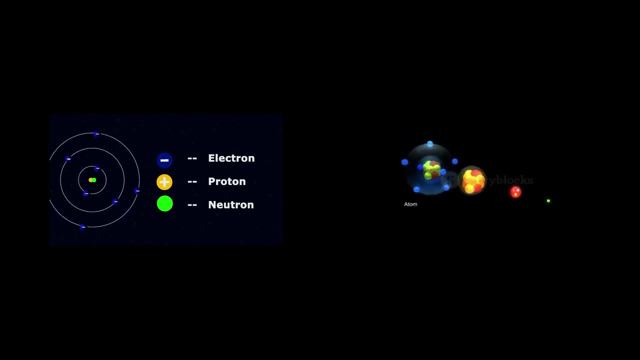 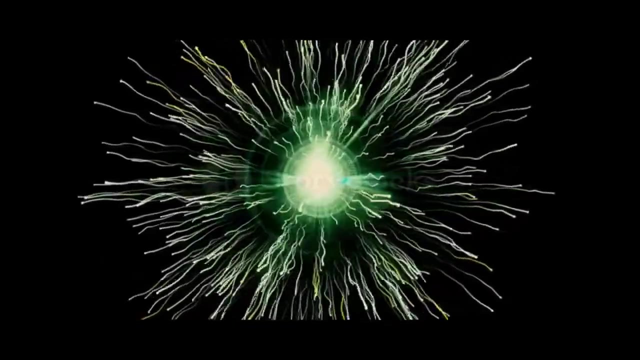 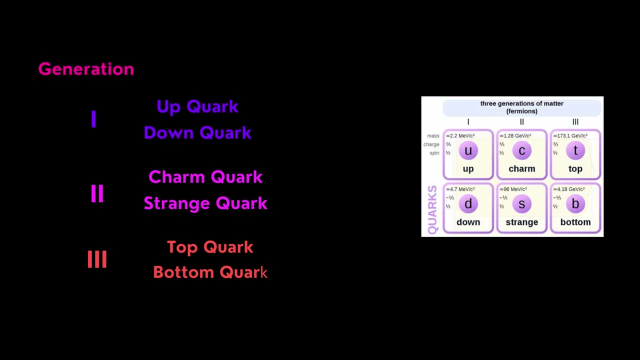 but were instead composed of smaller, more basic particles called quarks. This theory was later confirmed by experiments at particle accelerators such as the Large Hadron Collider at CERN. Quarks come in six different flavors: up down, charm, strange top and bottom. 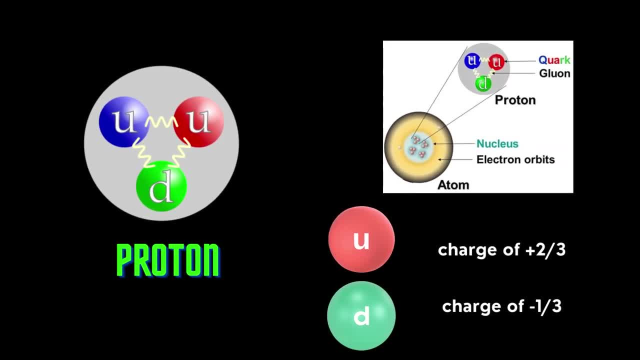 The most common quarks are up and down quarks, which make up protons and neutrons. Up quarks have a charge of plus two-thirds, while down quarks have a charge of minus one-third. These charges, along with the strong force, hold the quarks together in the nucleus of an atom. 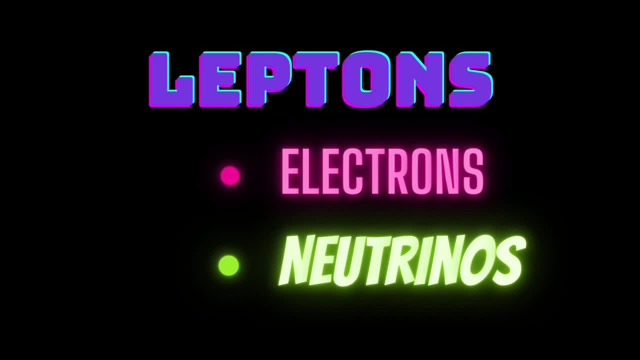 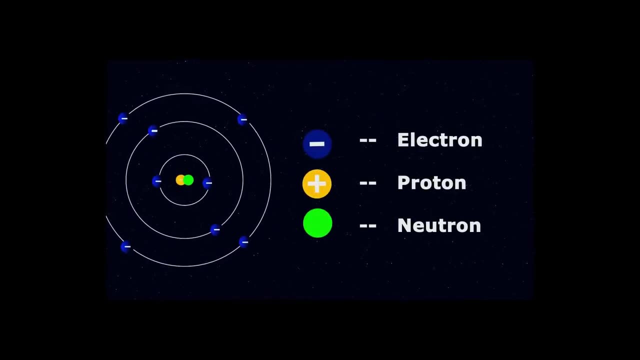 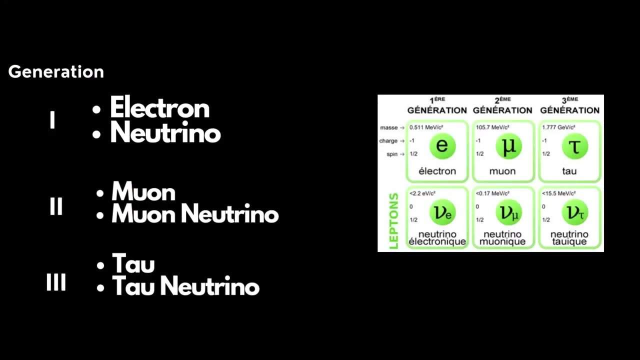 Leptons are one of the two basic types of fermions in particle physics, along with quarks. They are fundamental particles that do not interact with the strong force which is responsible for holding the nucleus of an atom together. There are six known types of leptons: electrons, muons, taus and their associated neutrinos. 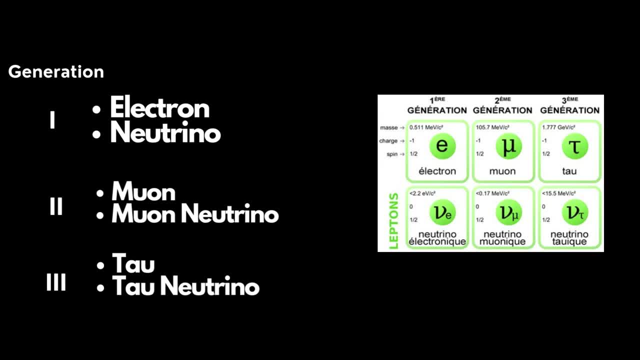 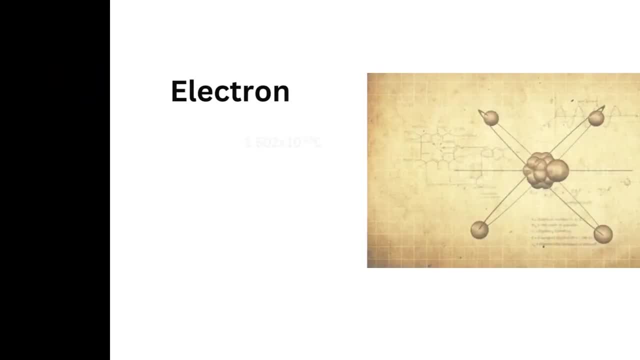 electron neutrino, muon neutrino and tau neutrino Electrons are well-known particles that are responsible for electrical conductivity and chemical reactions in the matter. They are negatively charged and have a mass that is much smaller than that of other particles. 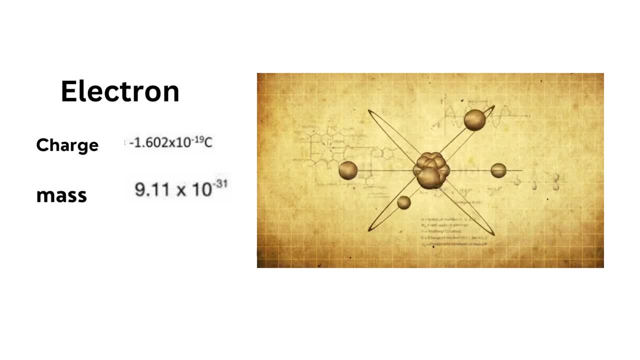 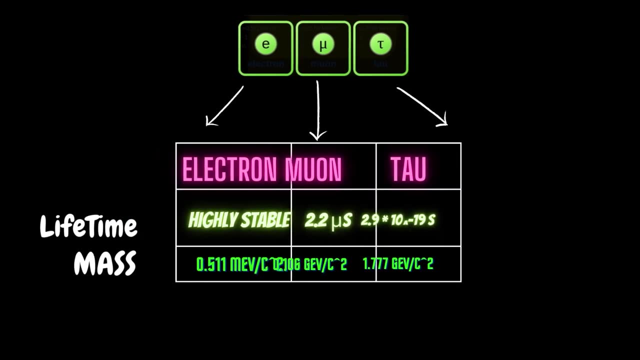 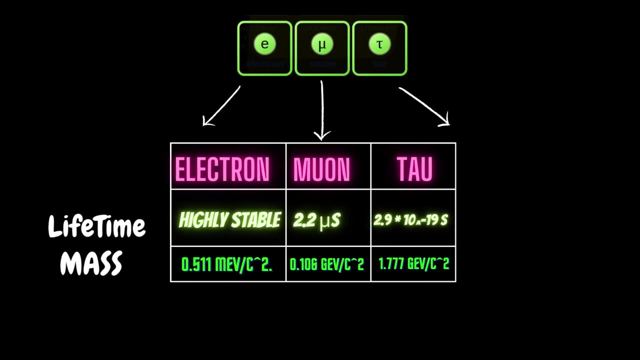 such as protons and neutrons. Electrons are considered to be elementary particles, meaning they are not made up of smaller components. There are three generations of electrons: parrot electron, electron, muon electron and tau electron. Electrons in different generations also have different lifetimes, with electrons in the first. 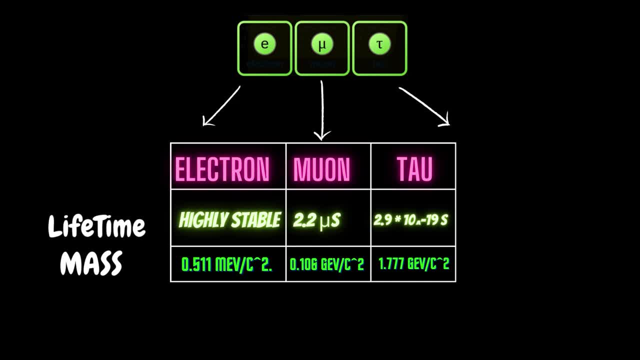 generation being the most stable and those in the third generation is the least stable. This is because the more massive the particle, the more prone it is to decay into lighter particles. Neutrinos, on the other hand, are much lighter particles that are nearly massless. 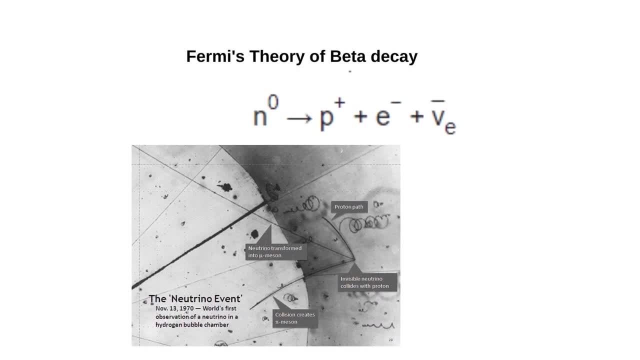 and interact very weakly with matter. They have a much vapor-dense response of about 5-7 mCa a minute on the glass surface and their pore density is about 3-6-8.5 MPa. They were first proposed in the 1930s to explain certain puzzling observations in nuclear physics. 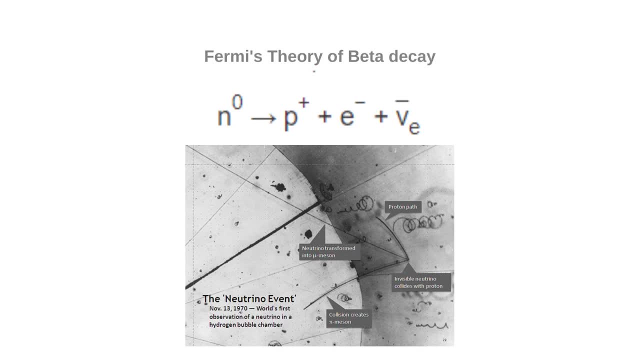 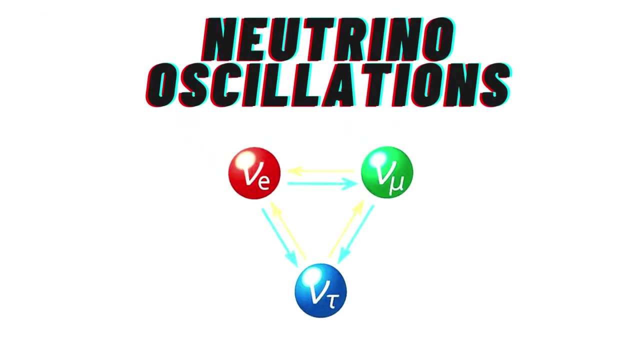 and have since been the subject of extensive study. Neutrinos come in three flavors- electron neutrino, muon neutrino and tau neutrino- and can change from one flavor to another as they travel through space, a phenomenon known as neutrino oscillation. 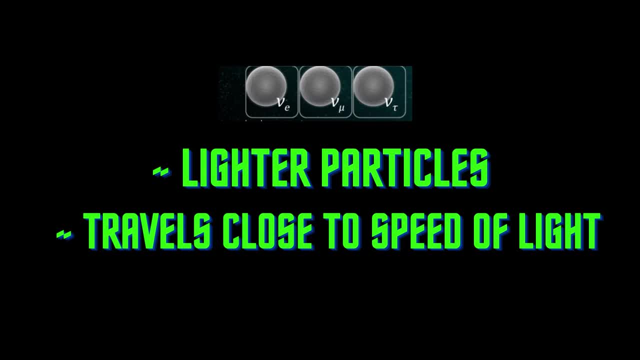 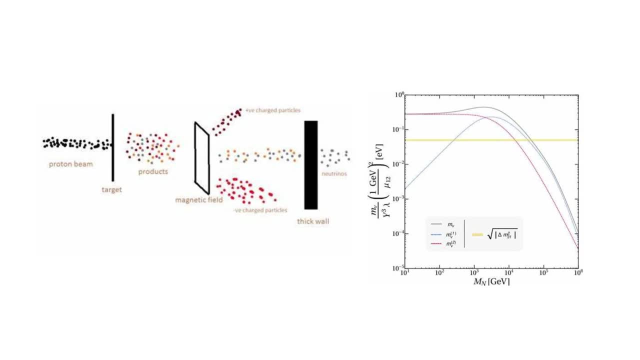 Neutrinos are interesting particles because they are very light and have almost no mass. They are also very weakly interacting and can pass through matter almost undetected. In recent years, the study of neutrinos has led to many important discoveries in particle physics. 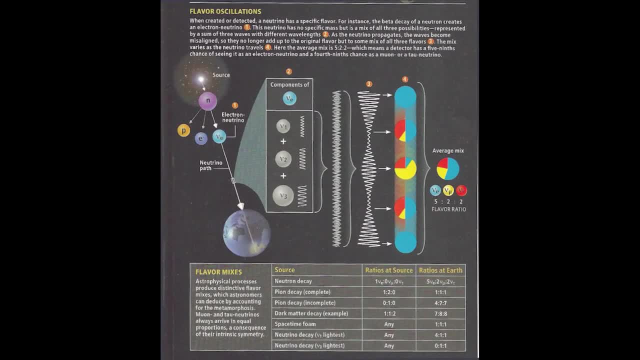 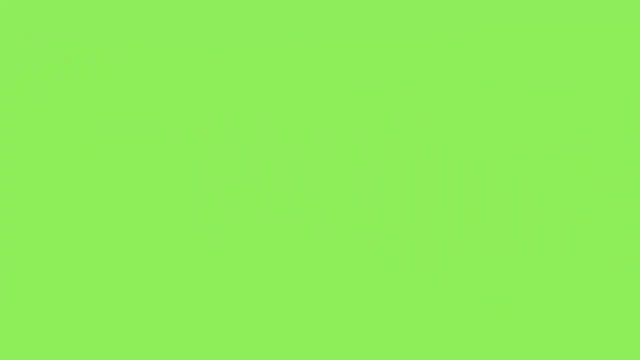 including the discovery of neutrino oscillation, which suggests that neutrinos have mass. Now let's talk about bosons. The bosons are responsible for transmitting the four fundamental forces: the electromagnetic force, the weak force, the strong force and gravity. 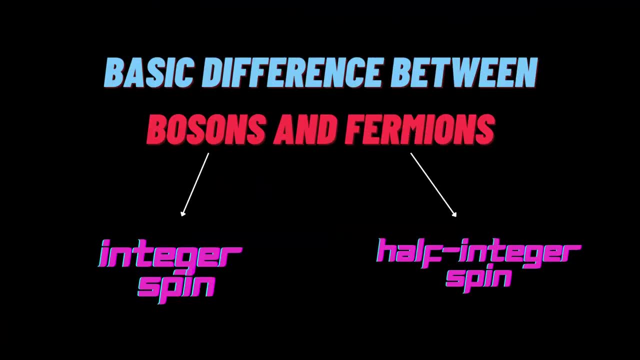 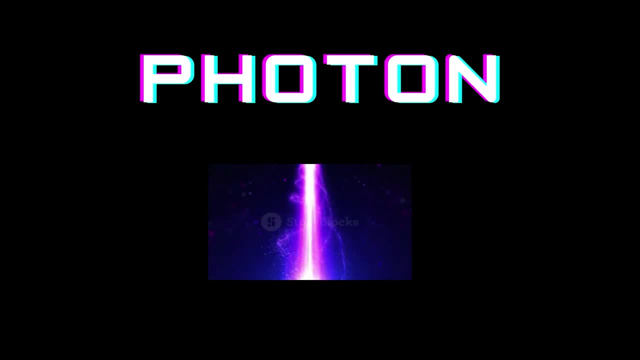 Bosons are particles that carry a force- of mass. They carry forces and have integer spin, while fermions are particles that make up matter and have half-integer spin. This distinction is not only about the particles, but also about the electrons. First we will talk about photons. 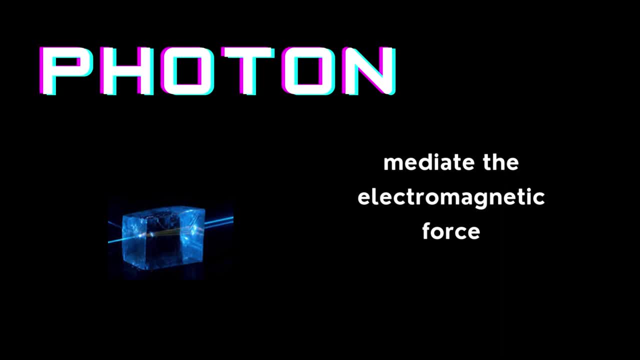 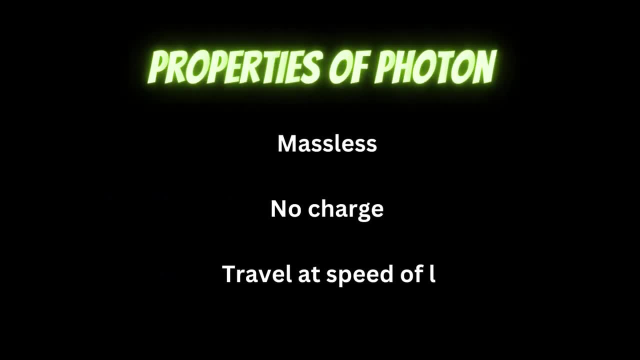 Photons are the particles that mediate the electromagnetic force, which is one of the four fundamental forces in nature. Photons are massless and have no electric charge, and they travel at the speed of light. They are responsible for transmitting light and other forms of electromagnetic radiation. 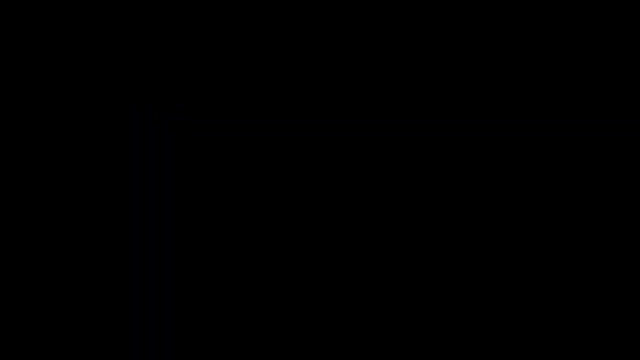 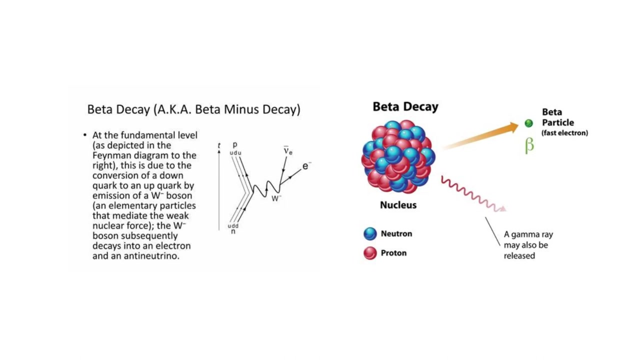 such as radio waves and X-rays W and Z bosons. The W and Z bosons are particles that mediate the weak force, which is one of the four fundamental forces in nature. The weak force is responsible for processes such as beta decay and other types of radioactive decay. 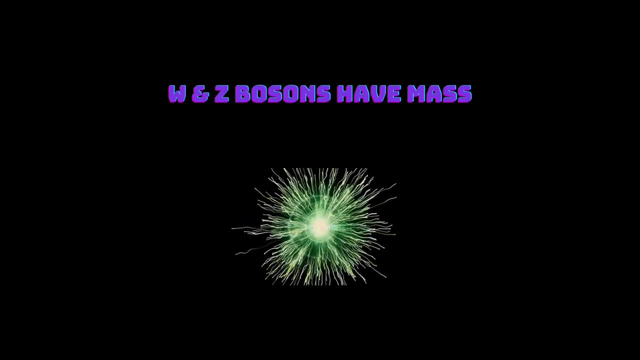 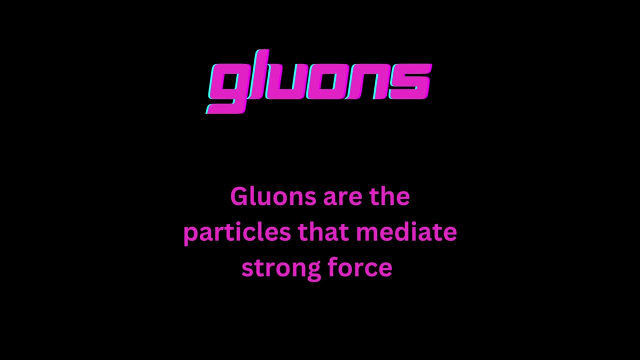 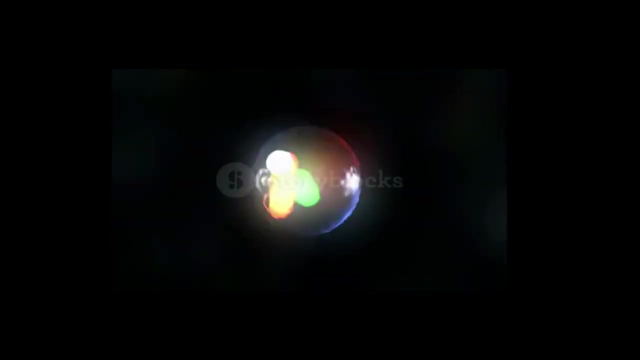 The W and Z bosons have mass and can be produced in high-energy particle collisions- Gluons- Gluons are particles that mediate the strong force, which is one of the four fundamental forces in nature. The strong force is responsible for holding the nucleus of an atom together. 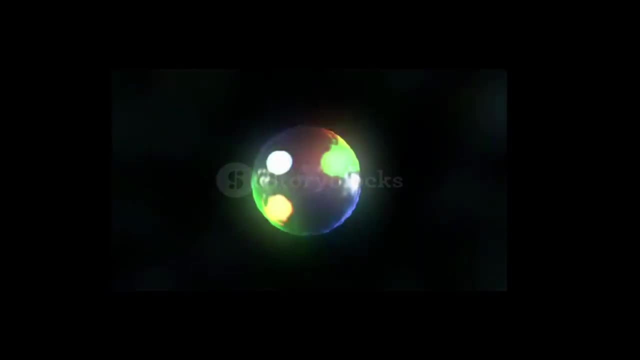 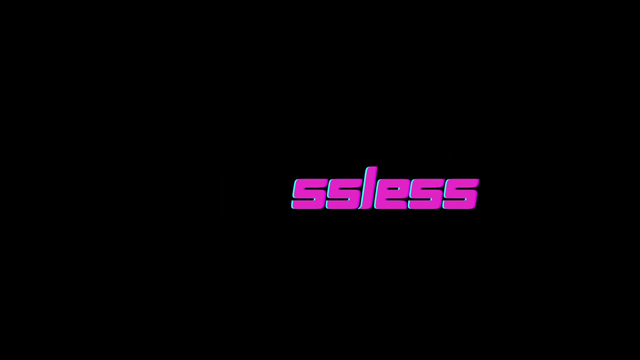 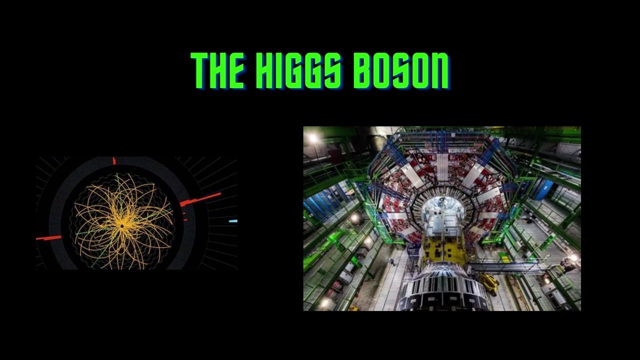 and is much stronger than the electromagnetic force. Gluons are massless and have no electric charge, and they are responsible for transmitting the strong force between quarks. Higgs boson. The Higgs boson is a particle that was discovered in 2012 by the Large Hadron Collider LHC at CERN. 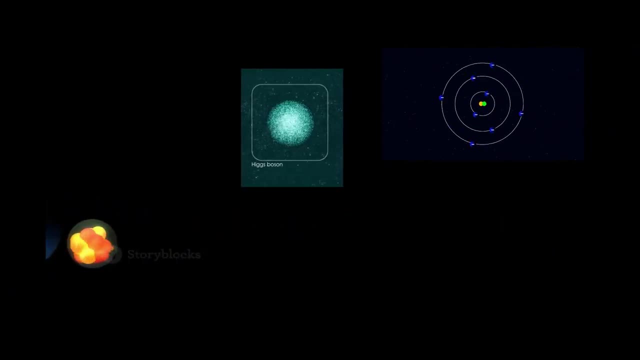 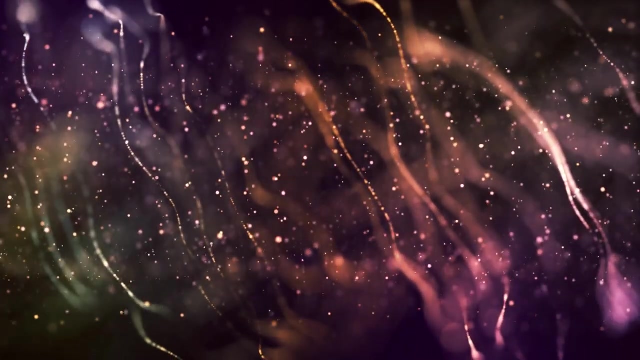 The Higgs boson is responsible for giving other particles mass and plays a crucial role in our understanding of the universe. The Higgs boson is associated with the Higgs field, which is a field of energy that permeates all of space and gives particles mass. These are the bosons that